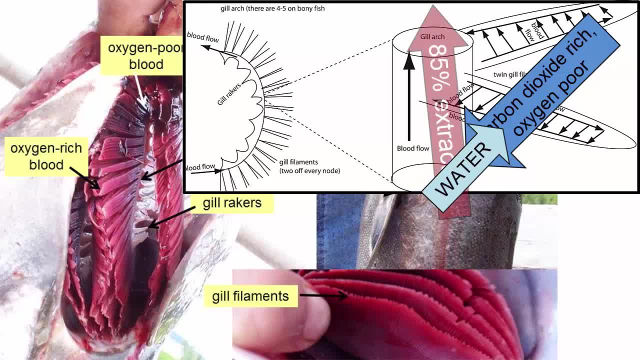 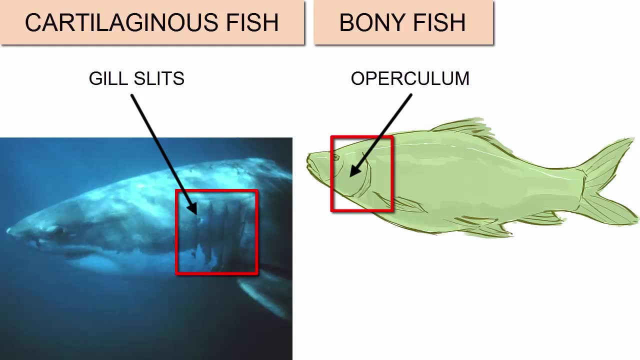 allowing maximal diffusion and extracting 85% of the oxygen. This blood is then circulated through the body of the fish for respiration and returns to pick up more oxygen as needed. Bony fish and cartilaginous fish can be distinguished by the presence of an operculum. 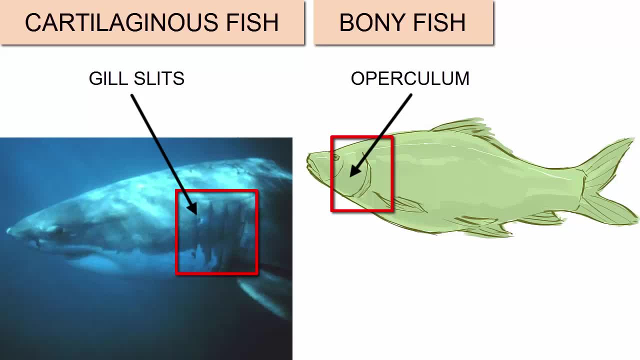 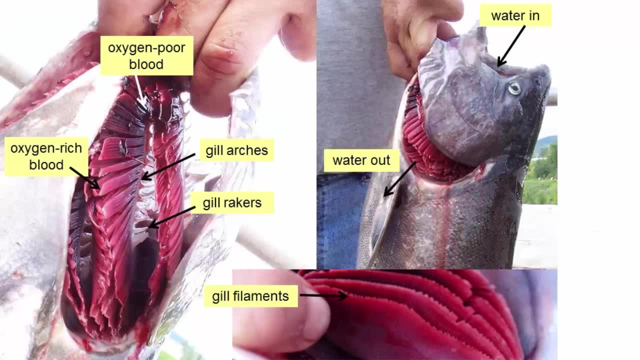 Most bony fish have one and it covers most of the gills. Cartilaginous fish have gill slits like portholes in the side of a ship. This picture of a Chinook salmon caught in northern British Columbia shows the individual gill arches. 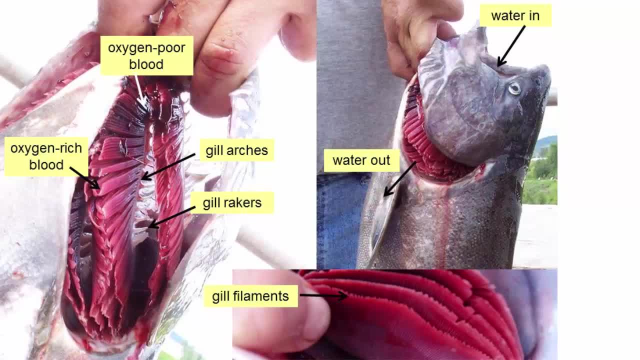 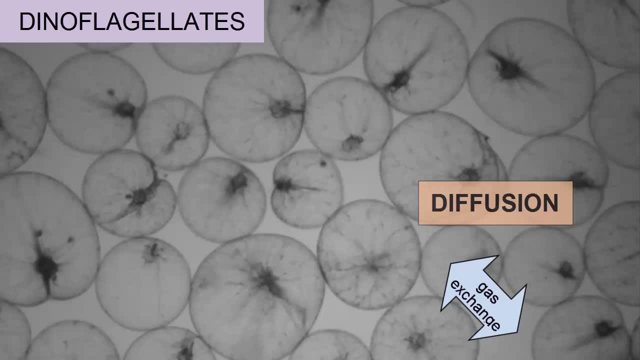 and filaments quite well. It also shows the path that water takes from the mouth through to the back of the operculum. Not only is diffusion an important process in gas exchange for all marine organisms, but it is also the primary mechanism for autotrophs to absorb nutrients. 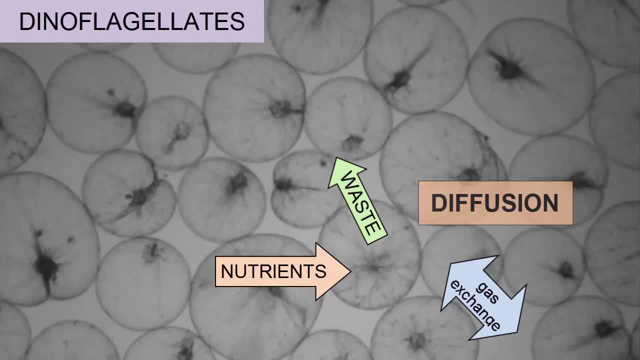 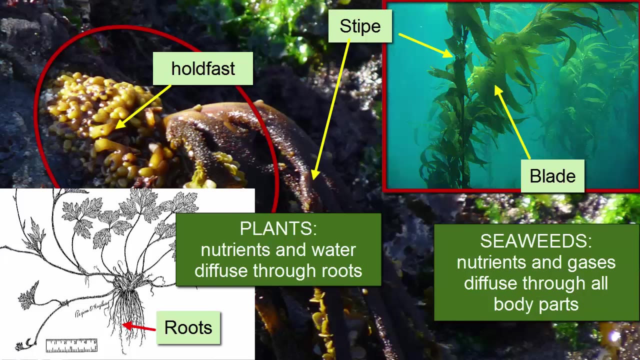 and for many organisms to eliminate their wastes. Seaweeds, sponges and all single-celled organisms in the oceans do most of their molecular exchanges through diffusion from and to the surrounding water. In fact, one of the major differences between marine autotrophs and most land autotrophs 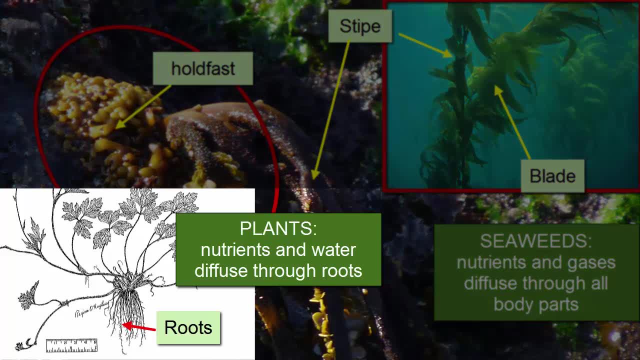 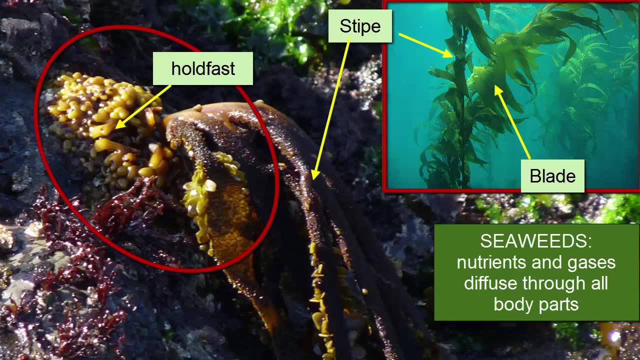 is that on land, autotrophs get their nutrients and water through diffusion through their roots, while in the ocean, diffusion can happen across all outer-cell walls at any part of the organism, including all stipes and blades on kelp and other seaweeds. 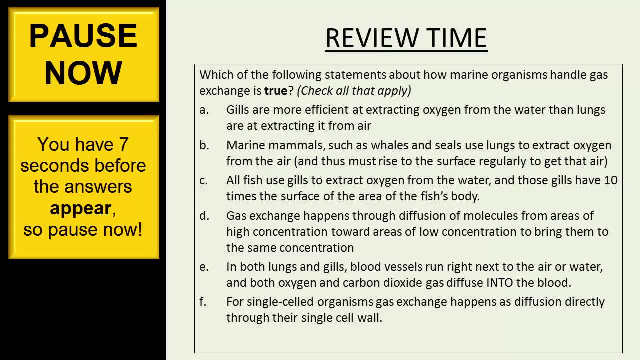 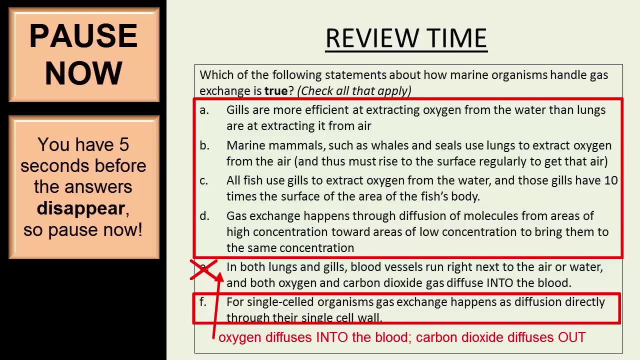 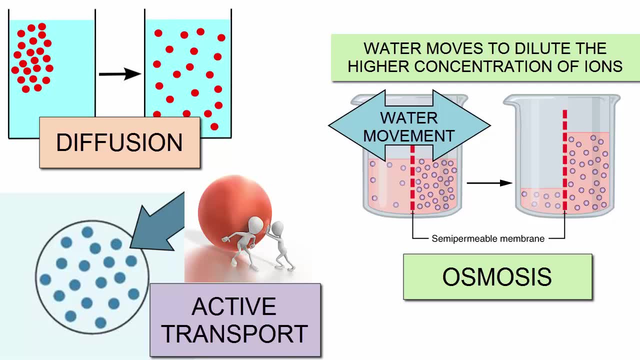 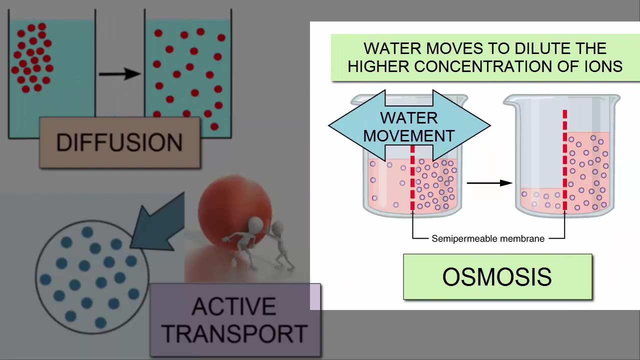 Pause now. This image shows three kinds of molecular transport, all of which are important to marine life. The top image shows diffusion, which we've already discussed. The middle image shows osmosis, which we'll get to in just a moment. 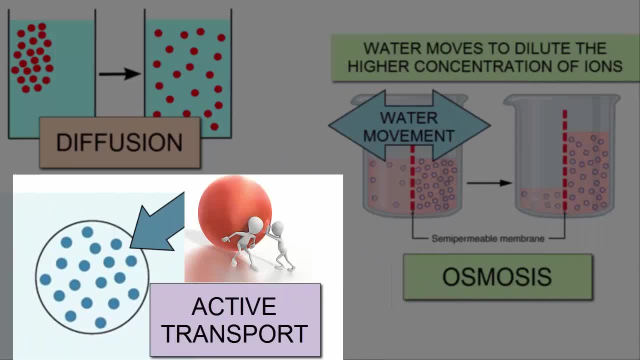 The final image shows active transport. You can see from this image that the concentrations of molecules are not the same on either side of the boundary. Such a situation is not in equilibrium. It must be constantly working against diffusion. It thus requires a lot of energy to maintain. 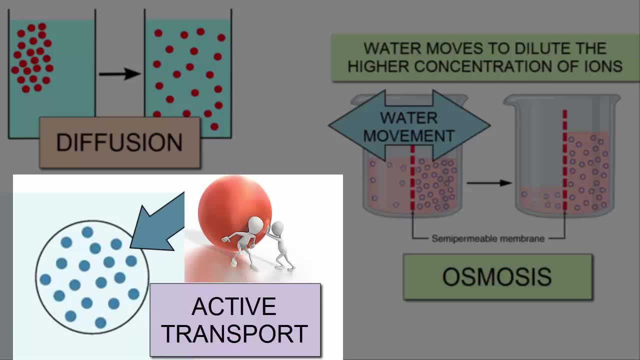 The boundary will open to transport the molecule uphill, so to speak, toward an area of higher concentration, but only if energy is provided to the system to make it happen. An example of active transport is what the body does when it stores fat in blubber. 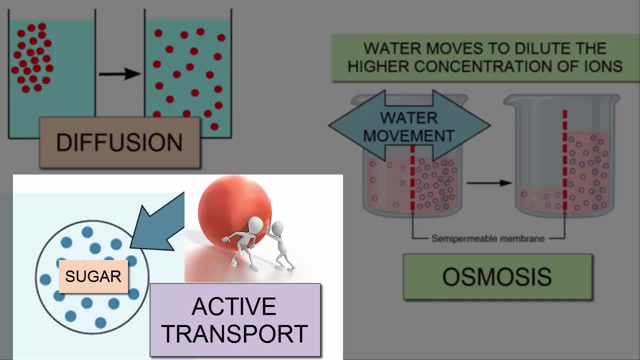 or other fat-rich cells, or when sugar is stored for later use. as needed, You can explore active transport processes further in a biology class. For now, it's sufficient to know that active transport requires an energy source and will not happen without it. 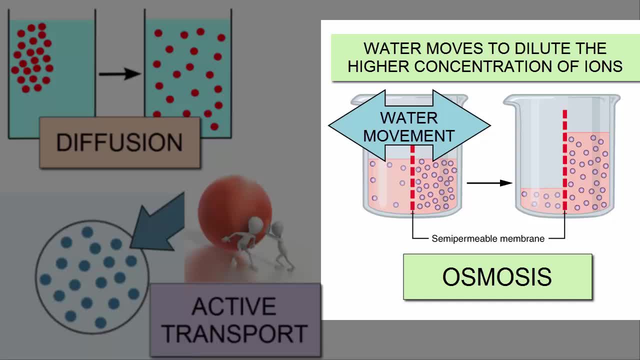 Now let's return to the middle image: osmosis. In this case, equilibrium is reached on both sides of the boundary, but because the boundary has holes that allow only water molecules through, equilibrium is achieved not by equal numbers of each molecule on both sides. 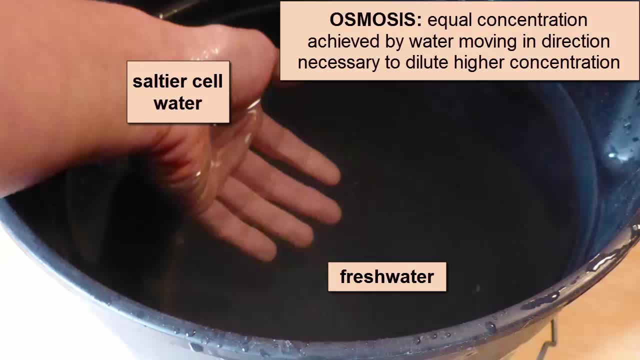 but by water moving toward the side that needs dilution. For example, here is a pail of fresh water. If you put your hands in this bucket, what will happen? Your skin cells will allow water to move across them, but not ions. 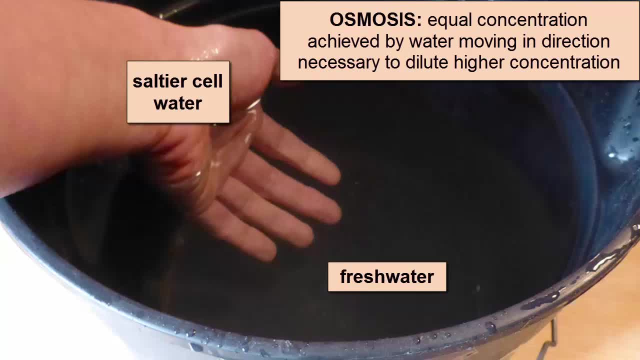 The fluid in your body is salty. If you've ever spent too long in the bathtub or swimming pool or hot tub, you know that the water will move across the boundary from the bucket into your hands, attempting to dilute the salty water in the cells of your hands. 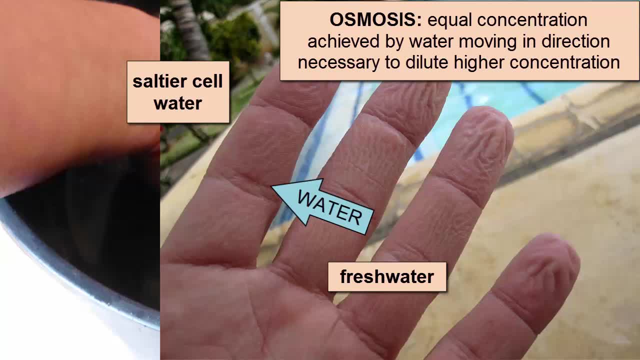 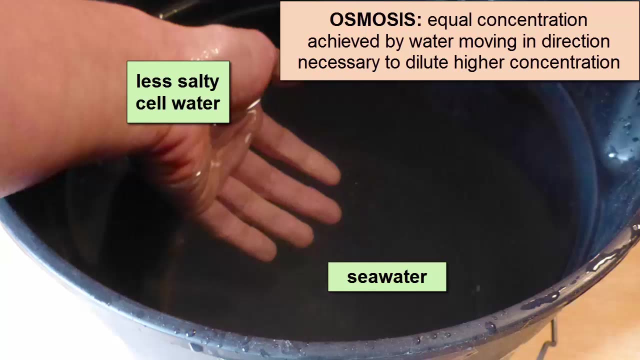 If you leave your hands in too long, they will swell up with water and the prune appearance results, which actually means your skin has swollen up larger than your fingers can contain it. What happens if the pail contains seawater? The salty fluid in your hands is not as salty as the seawater. 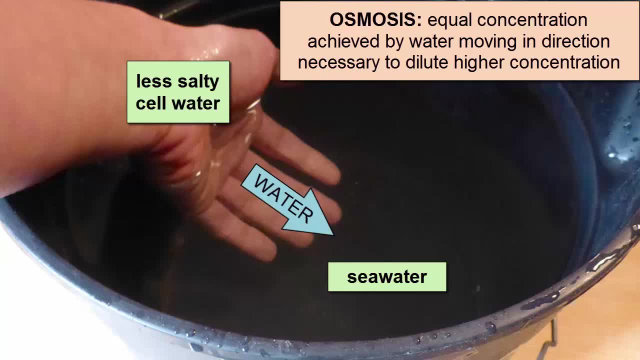 so the water in your body moves out into the seawater in an attempt to dilute it. Thus, after swimming in the ocean, your body will be dehydrated and you'll need to drink water to replace what you've lost. This is also why you should never drink seawater. 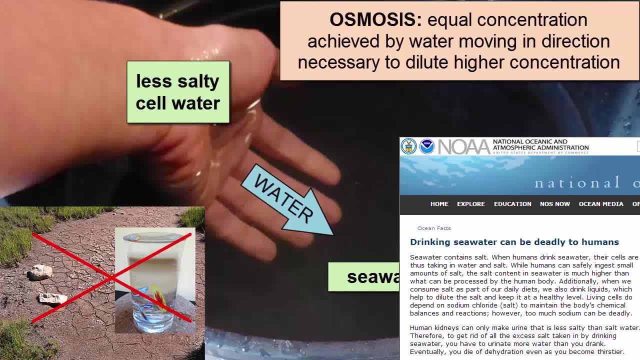 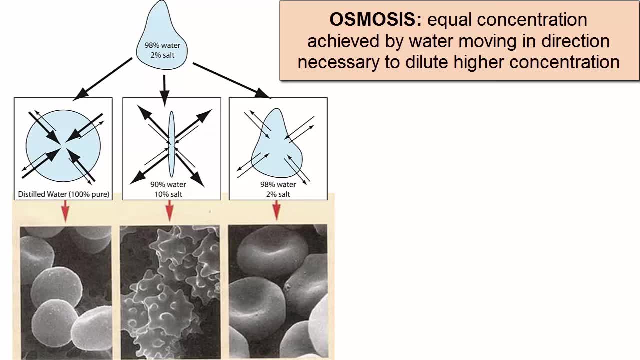 If you do, once it enters your body, it will draw out the water from the surrounding cells and you'll actually lose vital water from throughout your body. This image shows how your blood cells respond to osmosis. If your cells are like this bag and contain a salinity of 2%, 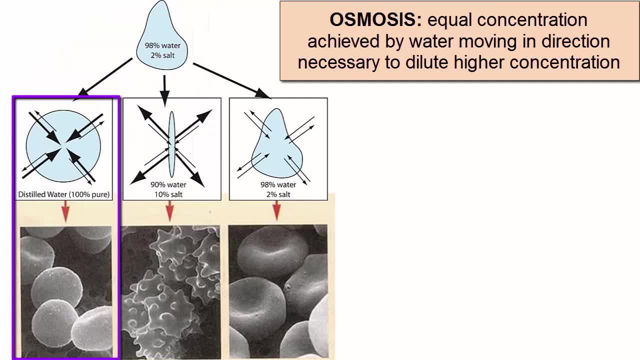 when you put them into a bucket of distilled water with no dissolved ions, water will move into the bag or cell to dilute the 2% solution inside. That means your cells swell up with water and can burst if the situation persists for too long.